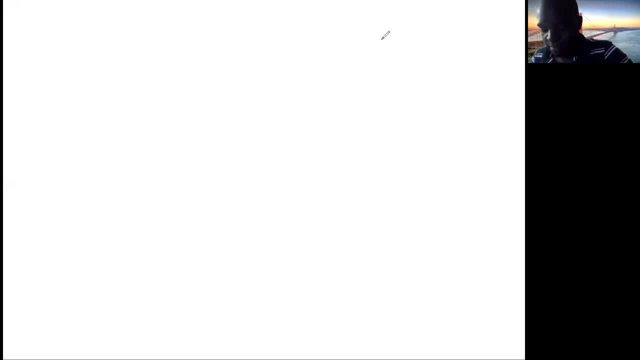 So we want to look at radical inequalities, Inequalities involving radical equations. So we are saying: inequalities involving radical equations. Okay, So we'll go straight into examples. Okay, So we'll go straight into examples. Okay, So we'll go straight into examples. 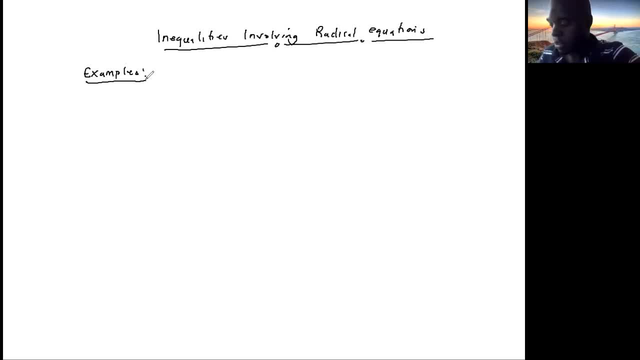 And this is Tereshit 6.. For some of you, it's Tereshit for the University of Zambia, And this is for you, Catherine, So A, so we're looking at question 3.. It's one that you're using as an example. 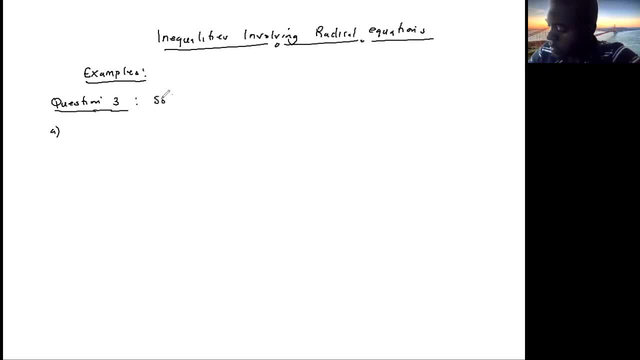 So the question is: solve each of the following inequalities: A 10 minus root of 2x plus 7 is less than 1.. Okay, It's less allowed to 3.. So the first that you do here is to move this 10 to the other side. 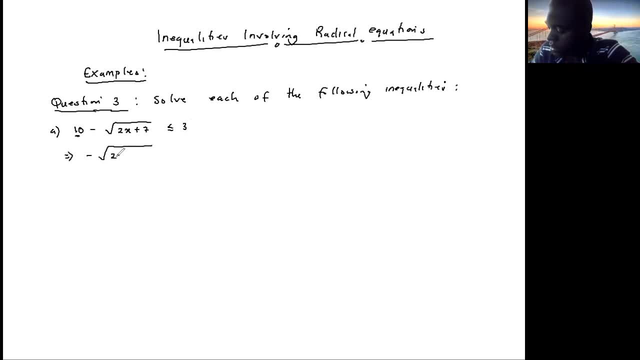 That implies that again to 2x plus 7 is equal to 3 minus 10, Which becomes negative 2x plus 7.. two x plus seven less or equal to negative seven, and then we'll have to square both sides. we have to square both sides. squaring both sides means that you've multiplied by the negative. 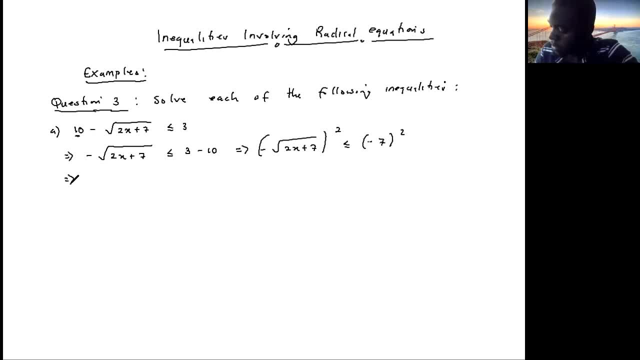 so it will affect the inequality. so on the left you're going to mean two x plus seven greater or equal to, so it quite changes because we have came back the negative that was on the other side, and so we have 49 on the right. so seven goes the other side. 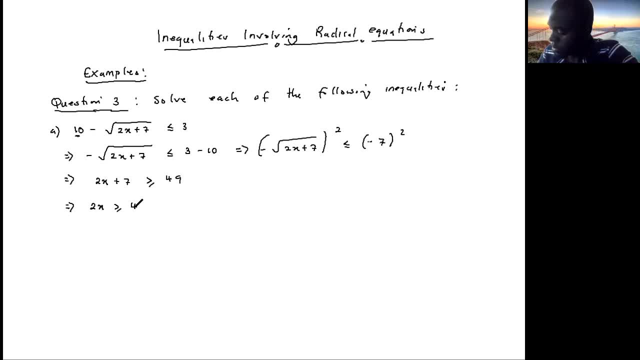 so we get 49 minus 7, which is 42. so when you divide by 2, we get x is greater or equal to 21. now you can test. you can test this is true. suppose you picked a number that is less than 21. let's pick a number like zero. 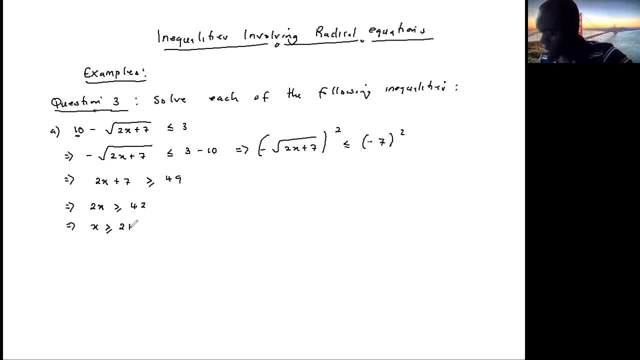 so let's pick a number like zero. zero is zero is less than 21.. so can zero satisfy this equation? so i'm going to have 10 minus seven. so this is indeed less. i go to three. is that true? no, so this is not true. okay, suppose you pick another number. 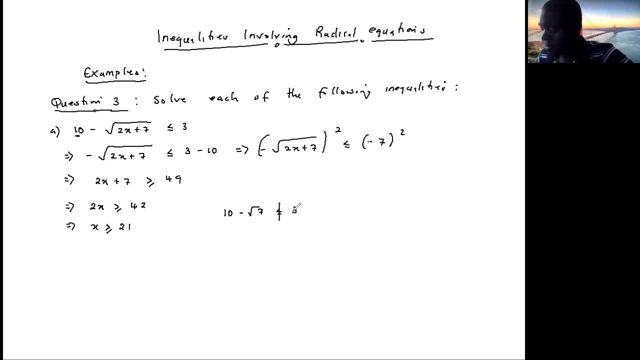 that is less than suppose you pick one. we're going to have ten minus two plus seven. this is ten minus root of nine, which is ten minus three, and this is not less than equal to. so it means that our interval satisfies the equation. so our solution, our solution set, is going to be one infinity and one. 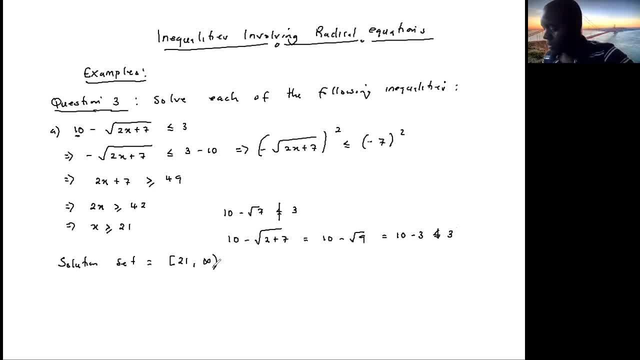 is included because we have less but equal to, or greater or equal. so look at the next question, B. so for B we have three less or equal to the root of 2x plus 5, and this is less than 6. so whenever we have this kind of inequality, 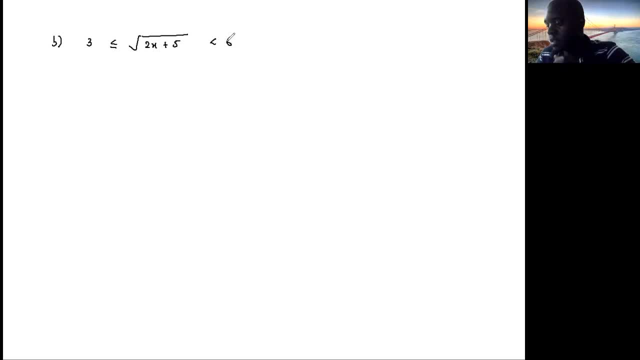 the radical is bounded. so it's, there's something burning it on the right and on the left. we can do it simultaneously by squaring all the parts. so we square this part, we also square the middle part, we also square the other part, so we have: 9 is less, or equal to 2x plus 5, which is: 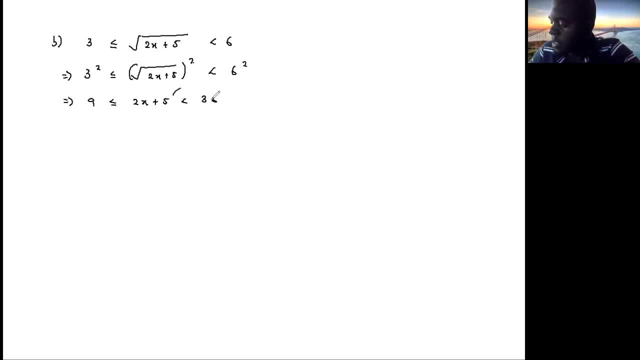 less than 36, then we take this 5 the other side, we also take the 5 the other side. in other words, we have less than 5 and we also take the 5 the other side. in other words, we subtract 5 from other three parts. so I have 9 minus 5, which is 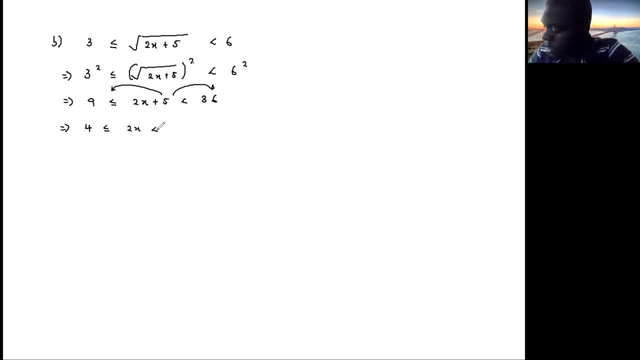 4 less or equal to 2x less than 36 minus 5, we get that one. then we divide by this to be divided by the 2, we divide by the 2, so you get 2 is less or equal to X, which is less than take one of a 2. this is a solution said so what happens is: 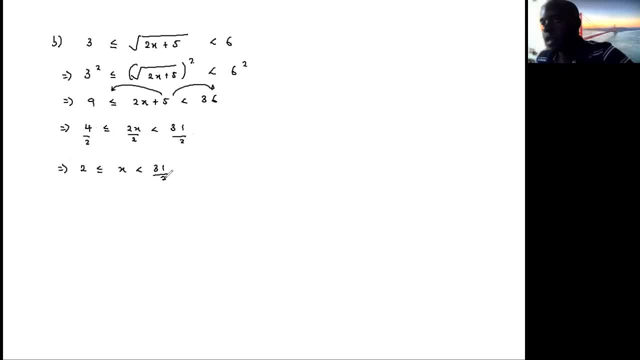 that you should do with radicals. for radicals, we always for squaring, because once we square, we have, then it means that we get rid of the radicals. so if, when you square once, you can't get rid of the radicals, you need to keep squaring until you. 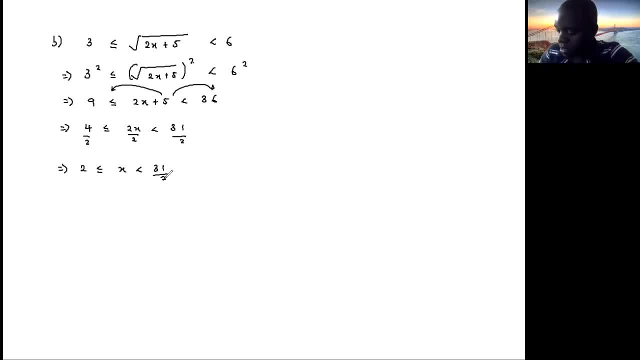 get rid of the radicals. that's the idea behind these types of questions. so i have c and that is 2x plus 9. minus 9 plus x is greater than 0. so if i take this- the other side, i'm going to have 2x plus. 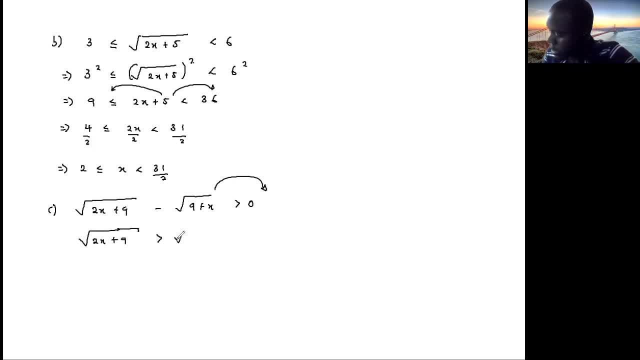 9 is greater than 9 plus x. so if we square this, if we square this, then what we get is 2x plus 9 is greater than 9 plus x. so if we take the 9 that side, we take the x this side, we are. 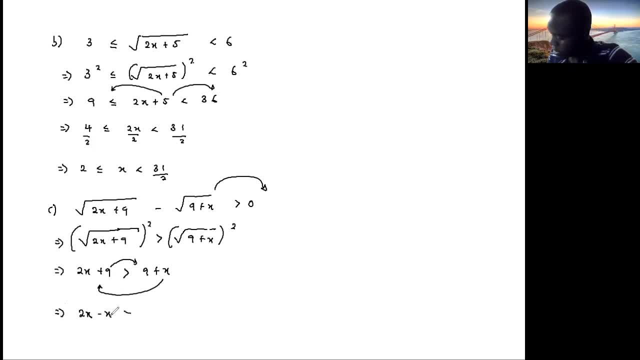 going to have 2x minus x is greater than 9 minus 9.. this implies that x is greater than 0.. so this becomes the solution set. so it's that nice and that easy. okay, so can it be another question d? so it has root. 2. 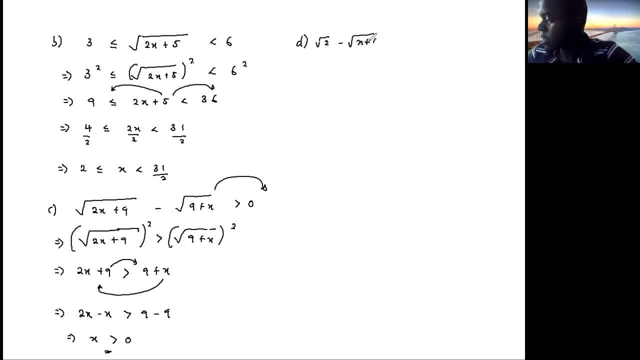 minus root x, plus 6 less or equal to negative root x. okay, so, by the way, this one has been first, we just start squaring wherever we are. okay, so we square the other side. we also square the left hand side, so we are going to get. 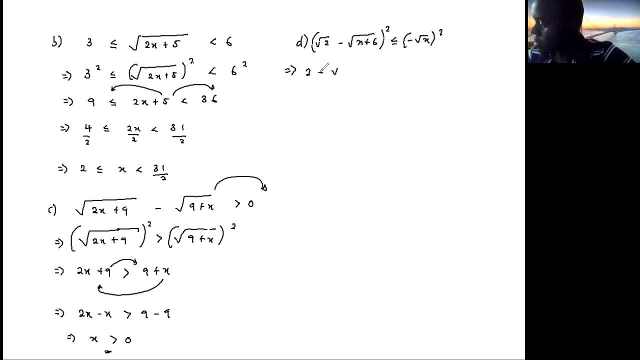 2 minus 2 by x plus 6.. so these are going to be two of them, because again we are still multiplying, and then plus x plus 6.. so this should be greater or equal to x. so i've changed the equality sign there because 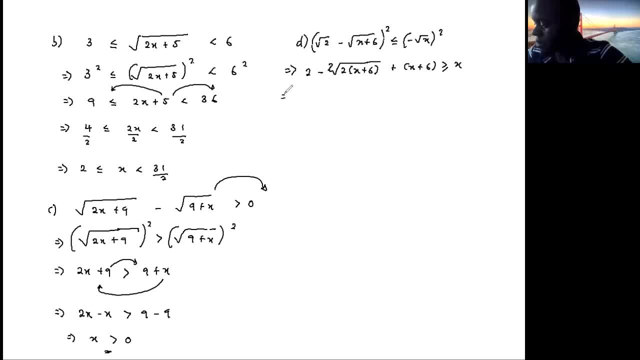 i've tempered the negative on the right so that we have 2 minus 2. root of 2x plus 12 is greater or equal to. so i can take this the other side, so that i have 6 negative 6.. so if we take this 2 as well, we are going to remain at negative 2 root of 2x plus 12. 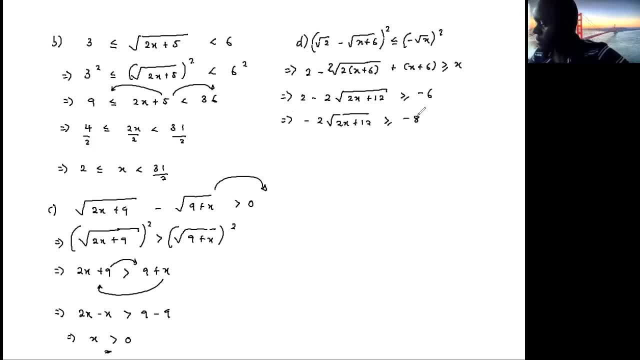 is greater or equal to negative 8. so if we divide by negative 2, we divide by negative 2 and we are going to have 2x plus 12 is less or equal to positive 4. so that if we square this side, we also square our side. 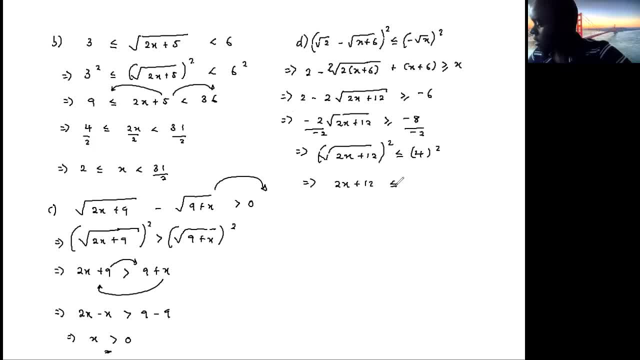 then we get: 2x plus 12 is less or equal to 16.. so you can take 12, the other side, so that we have: 2x is less but equal to 16 minus 12, we get 4.. so if we divide by 2, we divide by 2, x is less or equal to. 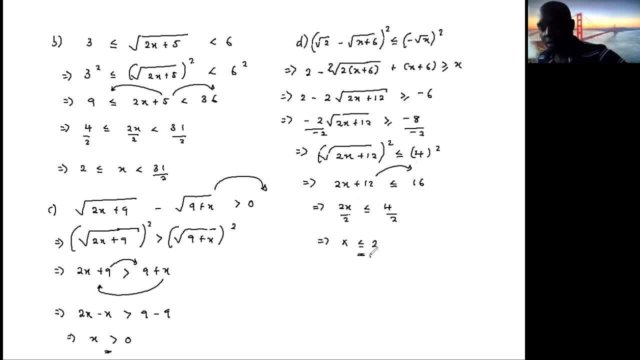 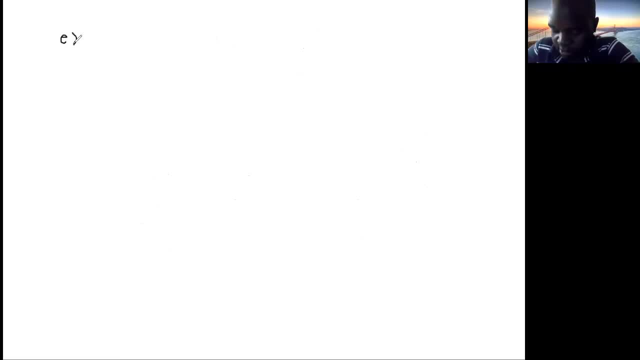 2 and this is the solution set. so it's this nice. so we do the last question on this part, that is x minus 3 greater than x plus 4 minus 1. so because of its nature, so we'll square the left hand side- we'll also square the right hand side. 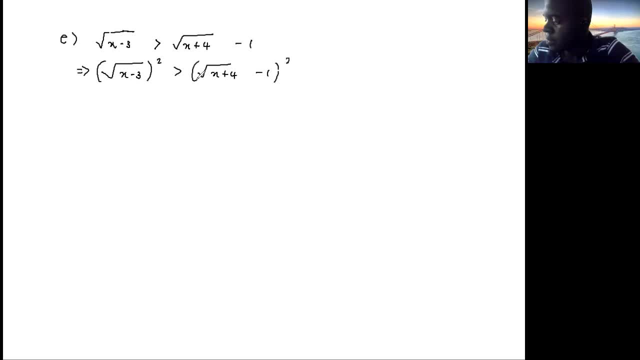 and i am going to divide it by 2x. so we have to divide by 2 x plus 4.. so minus 2 and plus 2 equals minus 2.. so we are going to have x minus 3 greater than x plus 4. 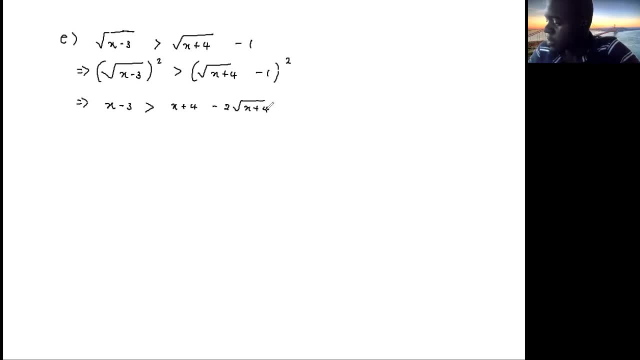 minus 2, x plus 4 plus 1.. so i leave the expansion part to be able to expand the power 2. that's not a big deal there. and then we take all this, we bring them the other side so that we have x minus x is going to be zero because now we're going to have x minus x. 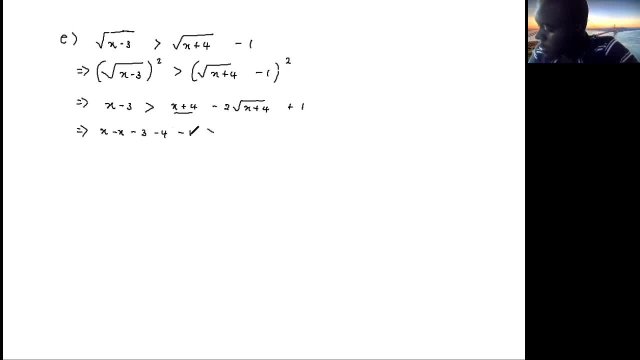 minus 3 minus 4. minus 1 is greater than minus 2 x plus 4, so that the x is disappear and so we have negative. h on the left is greater than negative 2 x plus 4. so if i divide by negative 2, divide by negative 2, what we get is 4 less than x plus 4. so when we square this part, 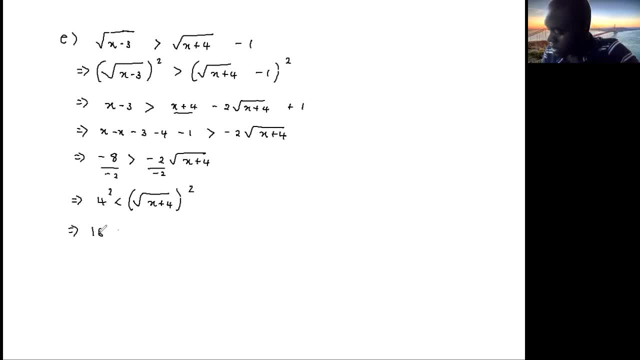 we also square the other side, so we get 16 is less than x plus 4. so notice how i change the inequality every time. i multiply the negative or divide by the negative, so that when this 4 comes the other side, we get 12 is less than x, and so the solution set is x greater than 12, which you can decide to write as: 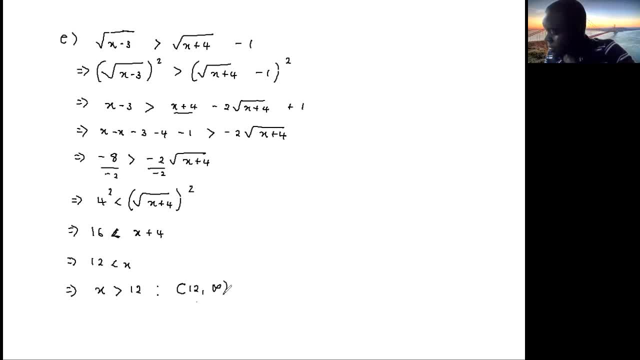 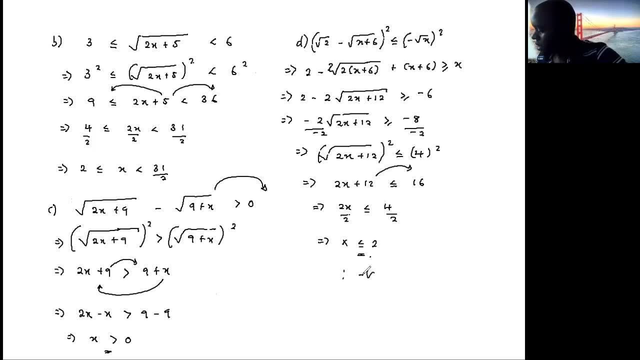 as 12 to infinity, so you can choose to write your answers in that form, so that you can write this one as negative, infinity to positive, 2 included, not included, and this one would be zero to infinite, like that, so that, um, this one can be two included.